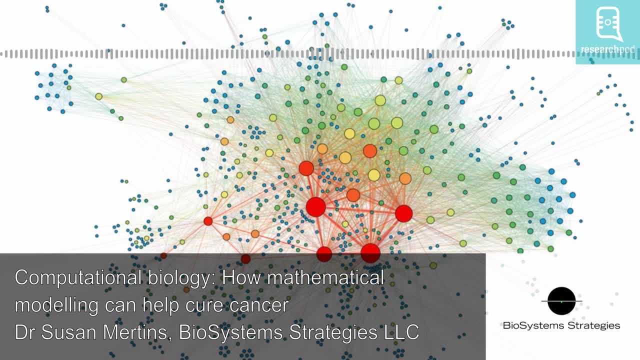 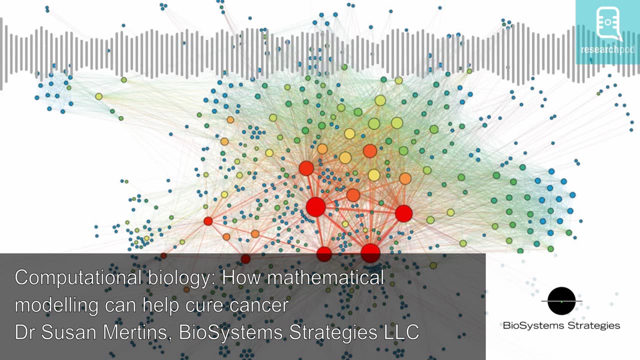 One approach is to use mathematical equations, the basis of computational modelling. Dr Susan Mertens, the founder and CEO of Biosystem Strategies in the USA, explores how ordinary differential equations and machine learning can be applied to cancer data for biomarker discovery and drug development, leading to improvements in personalised medicine. 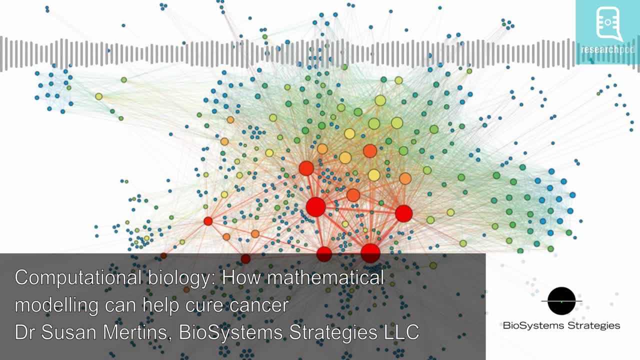 Biology. Biology is the subject of research. Biology is the subject of research. Biology is the subject of study of living organisms, which can be described as complex systems. Cells can have many different and sophisticated functions, for example, protein production and photosynthesis. 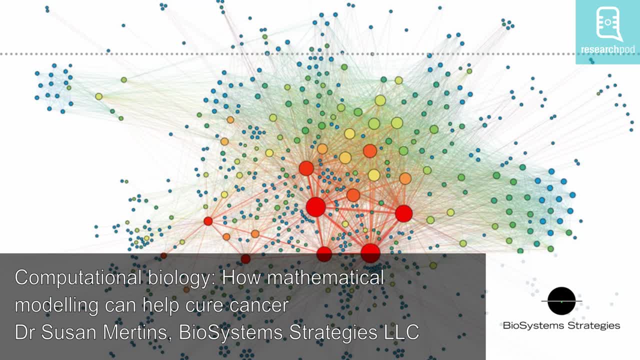 But because biological systems are dynamic and convoluted, this makes them challenging to analyse. However, specific mechanisms can be interpreted more easily using quantitative metrics. In other words, cell behaviours can be simplified by focusing on one specific aspect and only considering cell elements relevant to the question being asked. 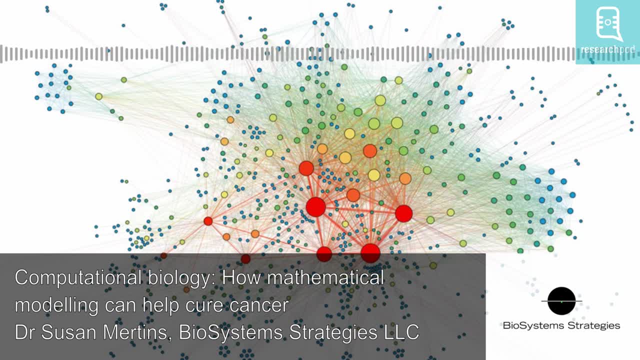 The biological phenomenon can then be approximated using mathematical equations. This is the principle underlying computational modelling, where biological mechanisms are represented using laws from physics and chemistry. Computational modelling enables us to simulate reality and make useful predictions in medicine, from drug development to biomarker discovery. 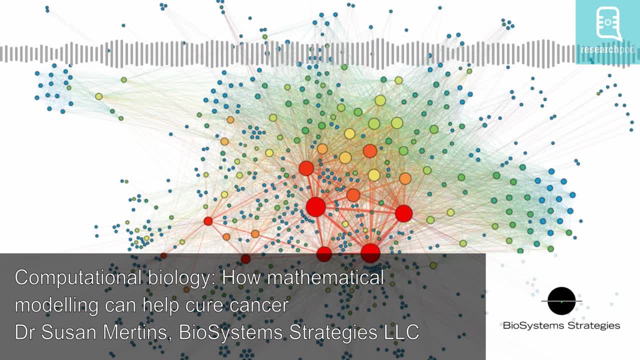 Dr Susan Mertens, founder and CEO of Biosystem Strategies, uses both computational modelling and machine learning to detect drug targets and biomarkers that will help develop personalised approaches to cancer treatment. The first step in computational modelling is knowing what you want to model. 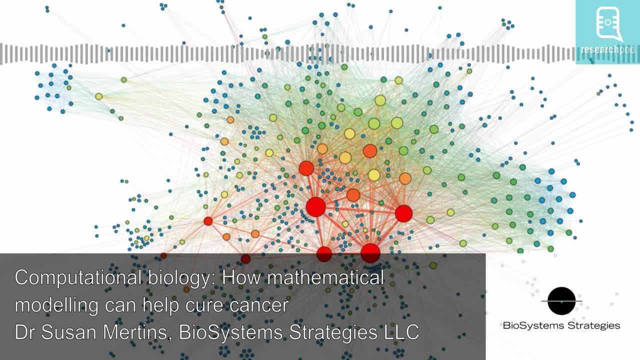 This may seem obvious, but being clear about this determines the choice of model and analysis. Following this conceptual phase, the actual model is constructed and the code for the simulation is written. While doing so, it's important to consider the role of the model in the simulation. 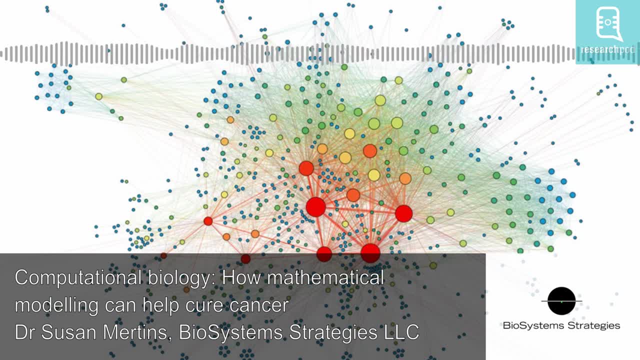 It's important to consider how the model can be verified by estimating the parameters and calibrating the model. As Musuamba and colleagues describe in a 2021 paper. verification can be seen as solving the equation in the right way, while the following step, validation, consists of solving the right equation. 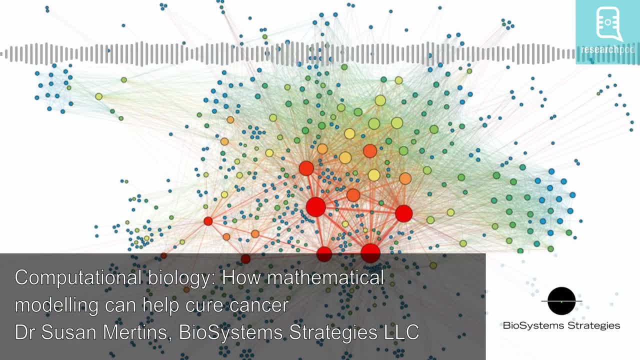 Model validation is the ability to simulate the conditions of interest, with certain sensitivities and uncertainties which reflect the quality of the model. Finally, the simulation is compared with comparator data to assess the credibility of the model, for example, using the results of a lab experiment. 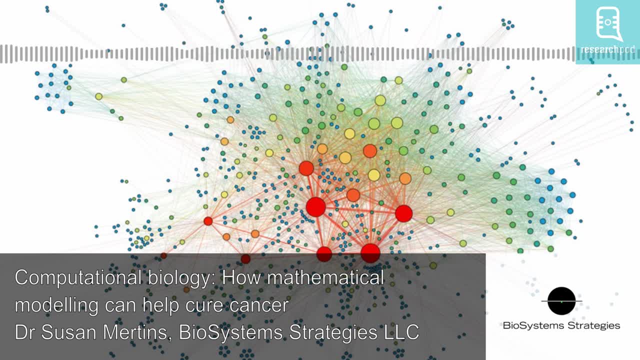 The type of model needed depends on the spatio-temporal scale of the biological process. For example, a reaction between enzymes will be faster than the development of a whole organ. The intracellular scale can be described with Ordinary Differential Equations, or ODEs. 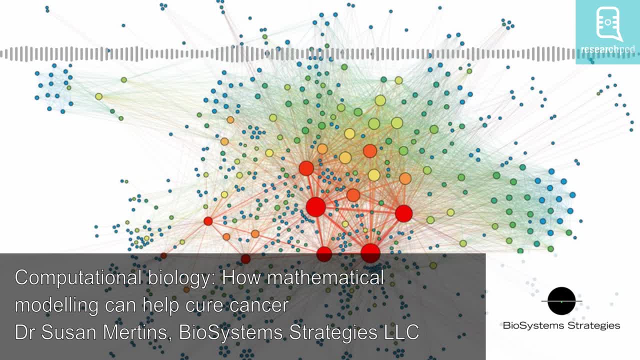 and involve a single variable that can describe a particle moving through a cell. Mechanisms such as protein gradients, however, are described by Partial Differential Equations, or PDE, which involve multiple variables and can therefore describe a surface changing over time. 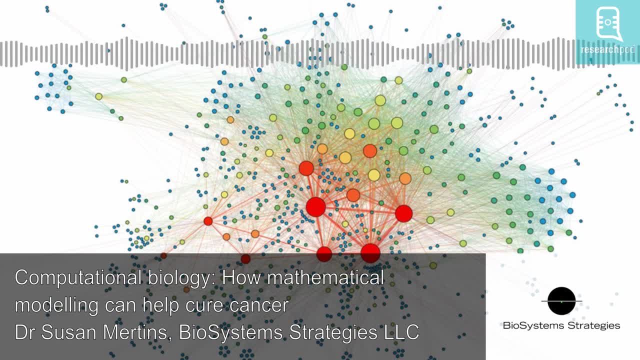 At the cellular scale. there are two main options of models, depending on whether space and time are considered discrete- known as on-lattice, or continuous, known as off-lattice. Agent-based models are a typical off-lattice model used to describe the interactions between individual elements of the system. 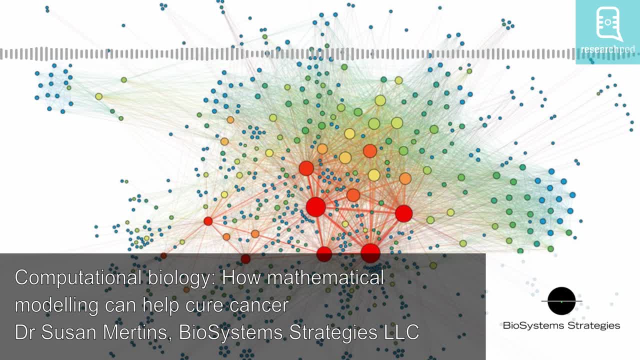 On-lattice models can be separated into two main categories: cellular automata, whereby agents are represented by a single pixel, and cellular POTS models, where agents are a collection of pixels. In other words, collective as well as individual cell behavior can be simulated. 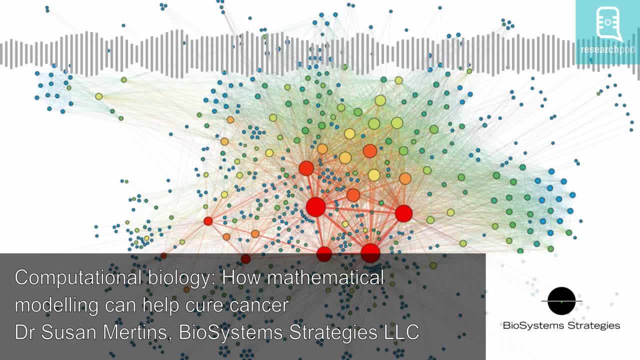 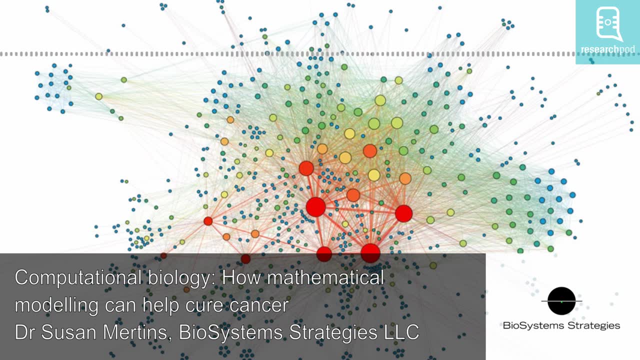 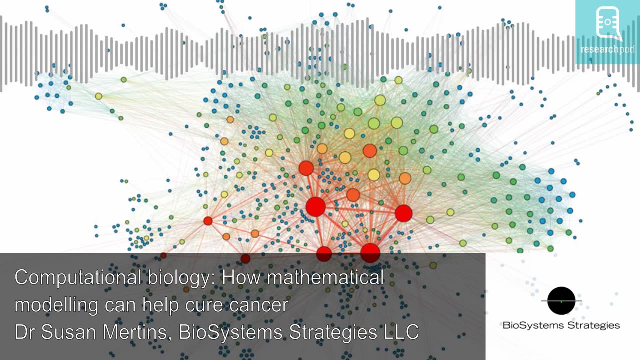 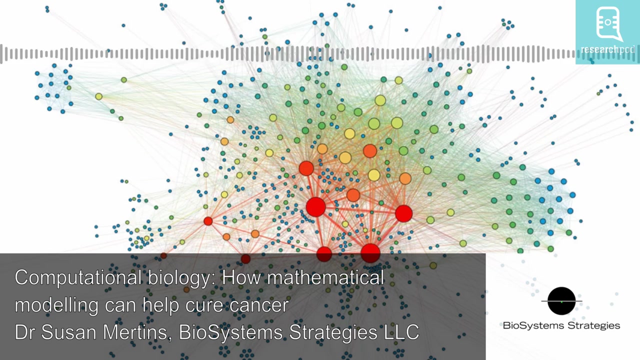 Cellular POTS models can therefore provide a greater resolution but are more computationally expensive. Whole cell modeling can be used to incorporate the different scales of a biological system and consequently predict how observable traits will arise from genetic mechanisms. Cancer is a complex disease which is hard to treat because of its heterogeneity. 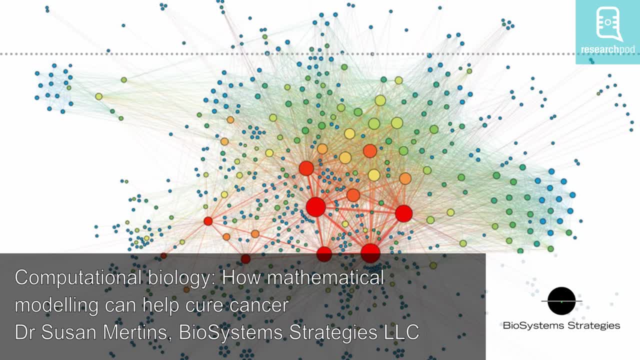 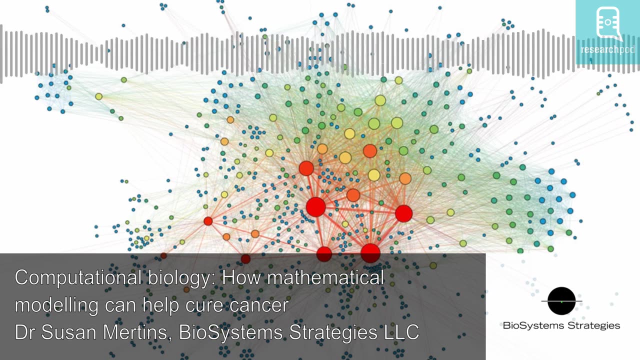 Different patients have tumors with different mutations, and even cells from the same tumor can have different mutations. Treating a tumor is therefore challenging, because if some cells are resistant to a treatment, the tumor can recur. Patients also have different metabolisms, so react to each drug differently.